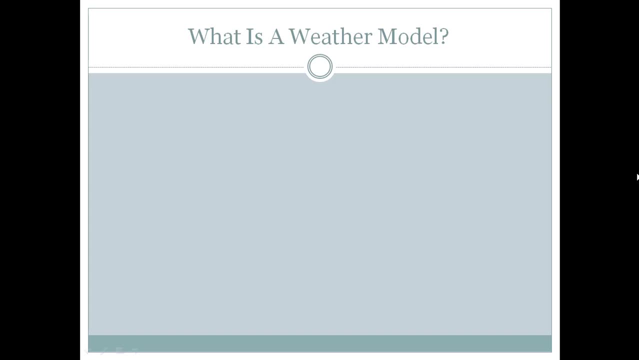 But first, what is a weather model? A weather model is a tool used by meteorologists in order to predict the future state of the atmosphere. There's a dozen of different weather models out there, each built slightly different from the other and built for different purposes. 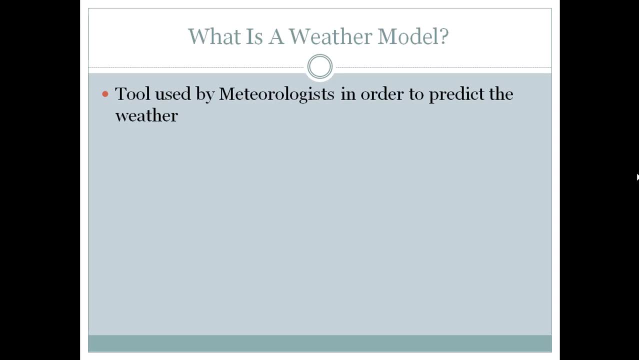 Some models focus on large-scale circulations of the atmosphere that are used for seasonal or long-term forecasting, while others focus on a more medium or short-range time span, like weeks, days or even hours. Weather models are dependent upon atmospheric data. 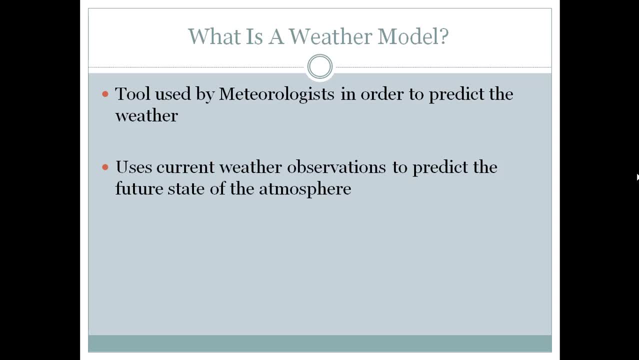 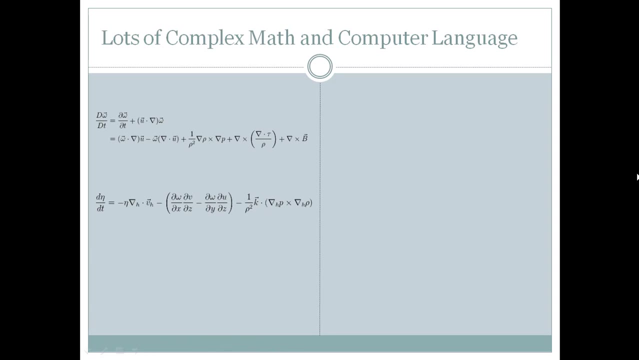 They take current weather observations and use that data to import them into the atmosphere. The weather models are then sent to these supercomputers that house the models, which then begin solving thousands of lines of equations that look like this and this: Meteorologists and computer scientists then take those complex equations and write them in code which the computer can then understand. 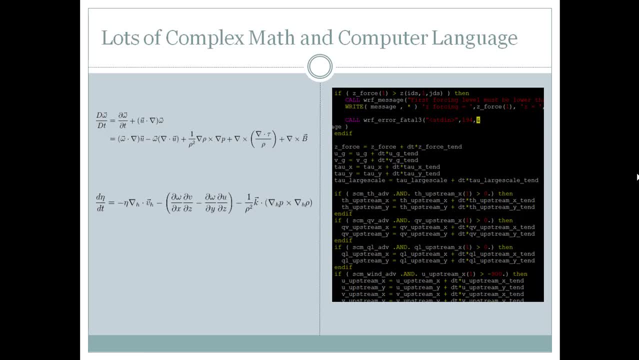 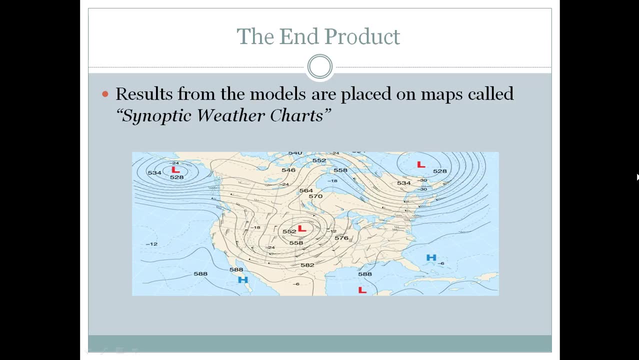 Eventually, the weather model finishes solving all those complex equations and outputs a result. The results are then overlaid on a map which is more visually appealing to the forecaster. So here's the weather model. He or she can then analyze the results and therefore make a prediction. 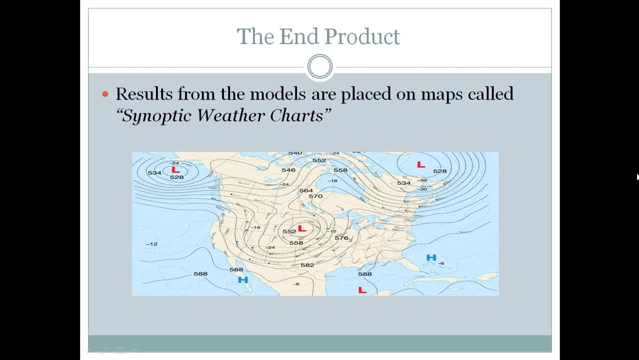 Since the results a weather model produces depends on the data going into it, oftentimes bad data will get ingested into the model and will then therefore produce an off result. It's then up to the forecaster to decipher which model looks to be more correct, which is also why we have a variety of weather models to choose from. 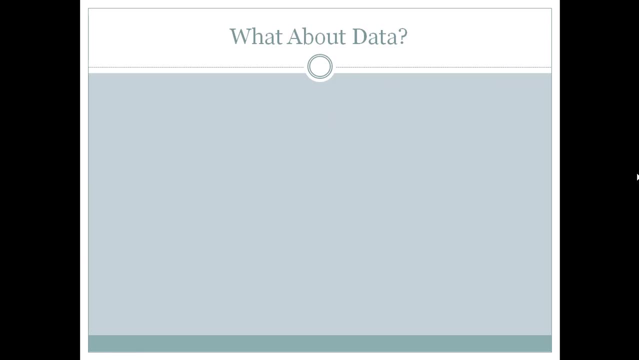 Now, this is a skill I will teach you down the road. Now, how do we collect data? While it's easy to measure things like temperature, humidity and wind speed here, at the surface, weather balloons are used to measure similar parameters aloft. 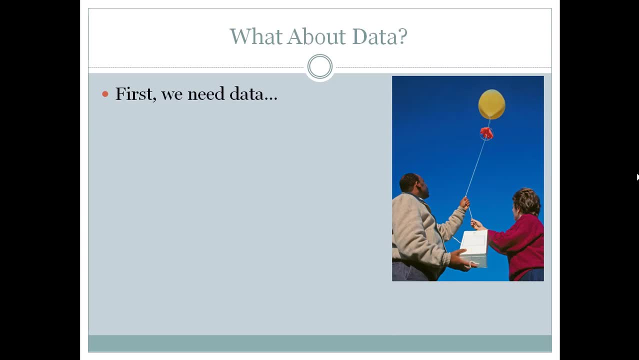 Weather balloons are launched at the same time around the world twice daily, both at noon and midnight. Attached to these weather balloons are instruments called radiosondes. Radiosondes also measure temperature, humidity, wind speed, direction and a few other key atmospheric factors. 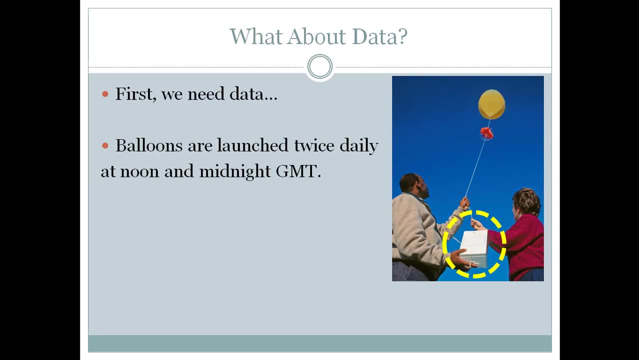 Those measurements are then transmitted back to the weather models that then begin solving those complex equations. The measurements give models key information on the current state of the atmosphere, so the model can therefore more accurately predict what might happen later. Each dot on this map shows where a weather balloon is launched. 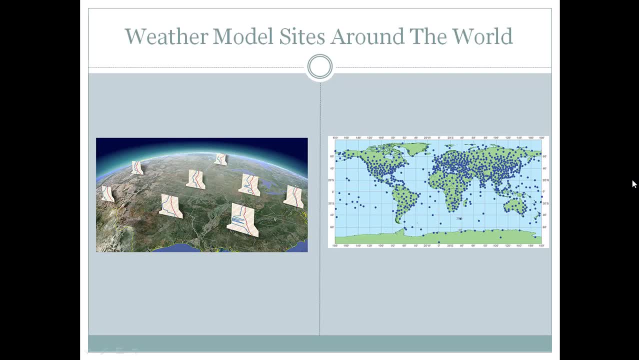 While there are a good chunk of locations that launch weather balloons, there's still a decent chunk of the atmosphere that's not launched, Simply because it's impossible for humans to measure every single inch of the atmosphere, which is why weather models sometimes produce bad results. 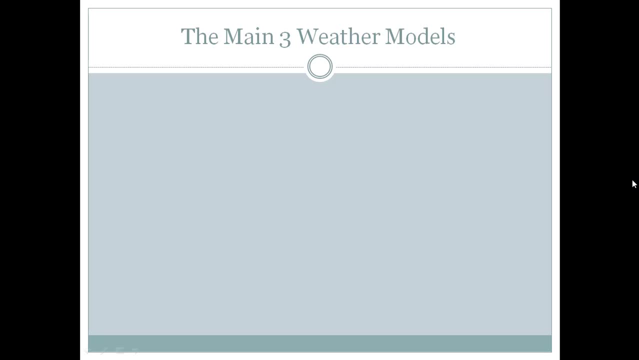 Now I want to talk about the three main weather models that you will see often throughout this course. The first one is the NAMM, which stands for the North American Model. It's an American-made model and it's more a short-range model, which means it only forecasts out 84 hours, which is only about three hours. 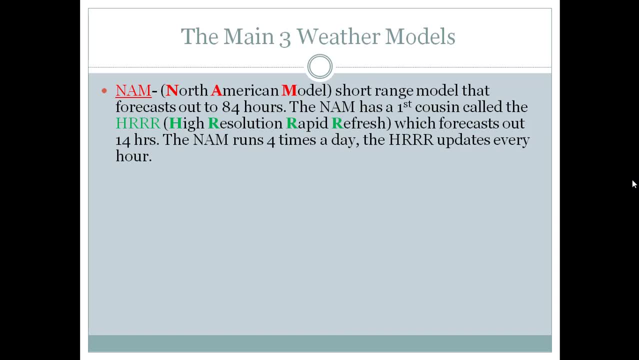 It's a short-range model. It's only about three and a half days. There's different versions of the NAMM, As I like to call them. they're the NAMM's first cousins. One of those cousins is the HER, or the High Resolution Rapid Refresh. 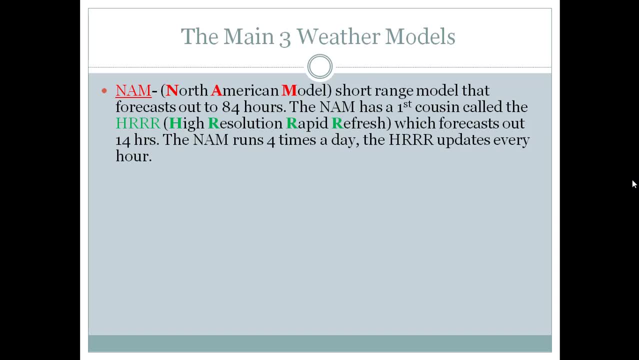 This is a very short-range model that forecasts out only to about 14 hours, While the NAMM runs four times a day. the HER will update every hour. Other versions of NAMM are called the WARF, which is used for research purposes. 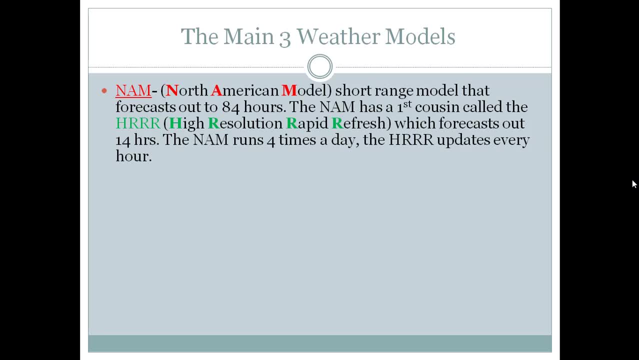 there's also what's called the RPM, which is more commonly used on TV, especially when they show the future cast of weather radar. The second weather model that we use often is called the GFS. It stands for the Global Forecasting System. 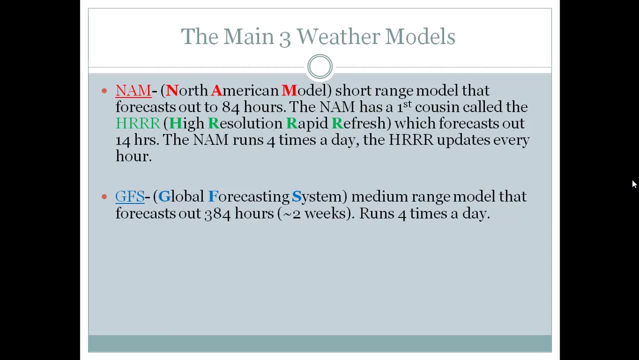 This is a medium-range model that will forecast out to 384 hours, which is about two weeks, And this also runs four times a day, and it's also an American-made model. Now, to compete with the GFS, we have what's called the European model.